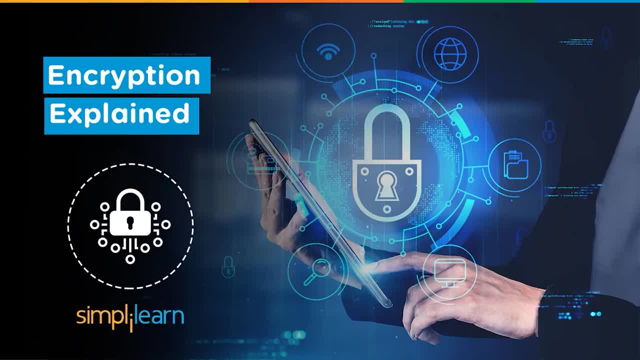 The fact that our browsing cookies have so much data to provide, all valuable information at that, is both alarming and a little reassuring, since our lives have become much more convenient. Either way, protection of this level of critical data is paramount, and encryption aims to do the same. 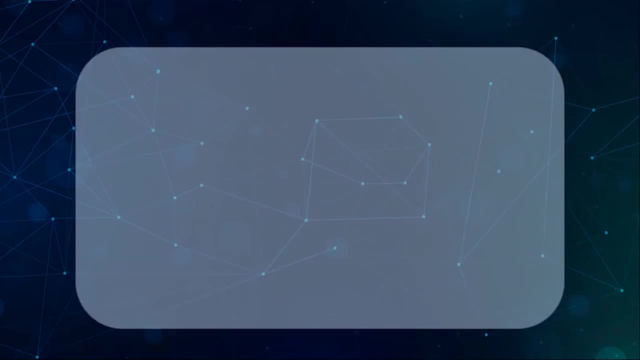 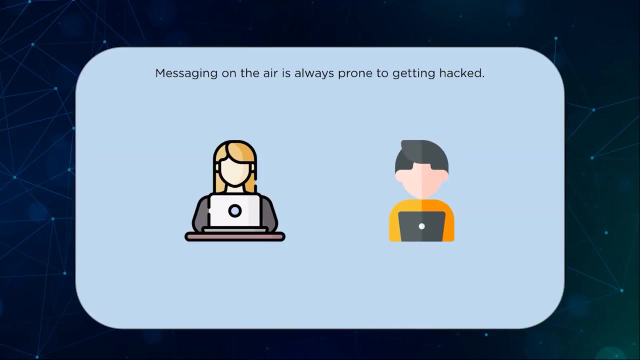 Let's understand why it's so vital in our digital world. A major portion of today's internet usage is the ability to chat on the air. We can send and receive messages easily. Messaging applications like WhatsApp, Telegram, Signal and many other transfer data over the internet, including our private messages, videos and 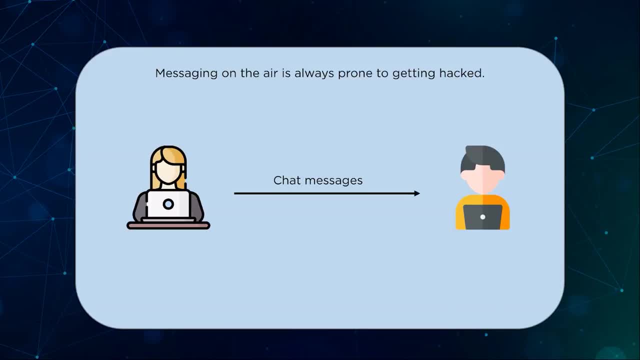 notes. In spite of repeated assurances, there is always a point of failure in the chain of communication. A dedicated hacker will only have a slaver of information to be able to crack into this channel and intercept all communication between users. This is where encryption comes into play. 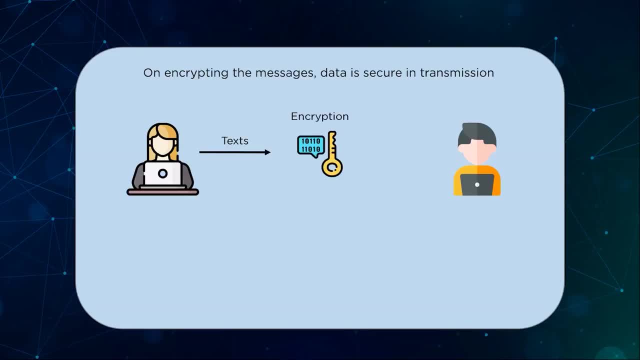 Instead of just transmitting the original message, we convert the message into a ciphertext. This is done by using encryption keys that apply mathematical calculations to the original information before it is transmitted. The scrambled information, which is known as ciphertext, is then sent to the receiver. 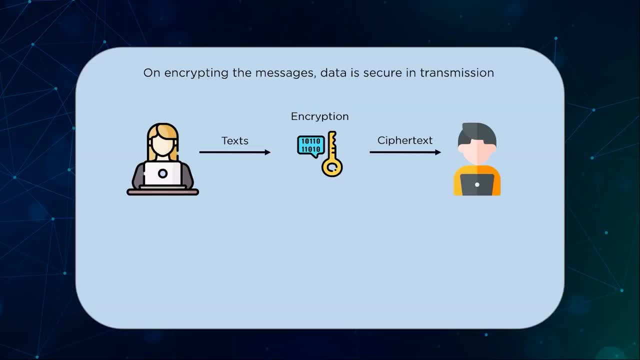 The receiver must possess a decryption key that may or may not be the same key used to encrypt the data. This decryption key must be settled with the sender before the messages are transmitted, or in modern messaging applications, the key management is done on the server side. 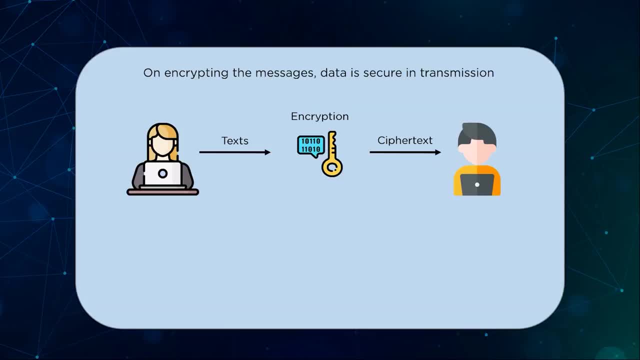 to benefit all users without compromising the security of the base platform. The advantage of this approach is that anyone listening to the conversation channel will not be able to receive the original message. Don't be mistaken: They can capture the ciphertext in transit, but they will never. 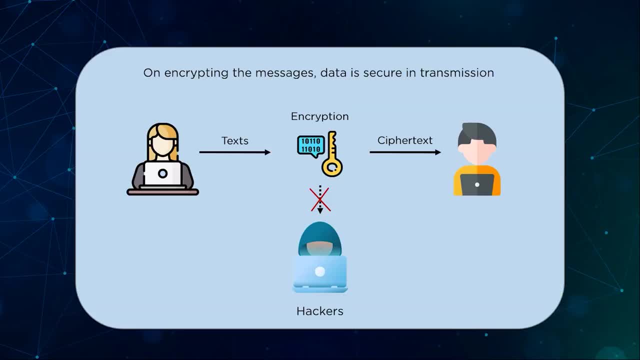 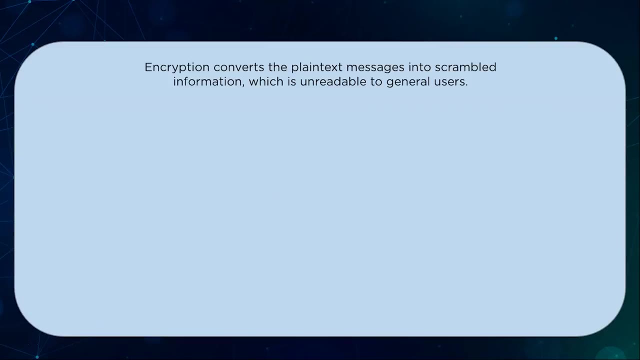 be able to decipher the original message without a decryption key, which only the specified sender and receiver have access to. But how does one go about this process? Let's know what encryption does with our messages. All of this encryption and decryption falls under the blanket of cryptography. Cryptography. 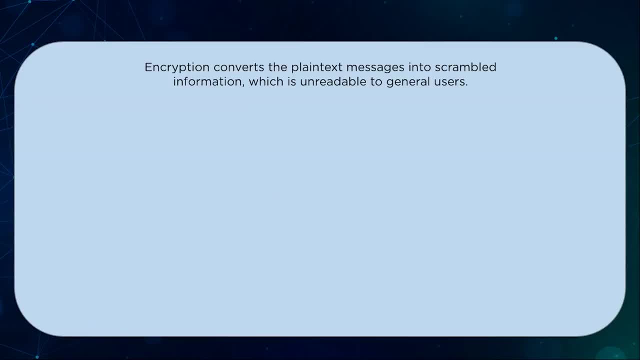 is the science of encrypting or decrypting information to prevent unauthorized access. We transform it into a decrypting system, We transfer the encrypted information to the server and then we transform our data and personal information so that only the correct recipient can understand the message. 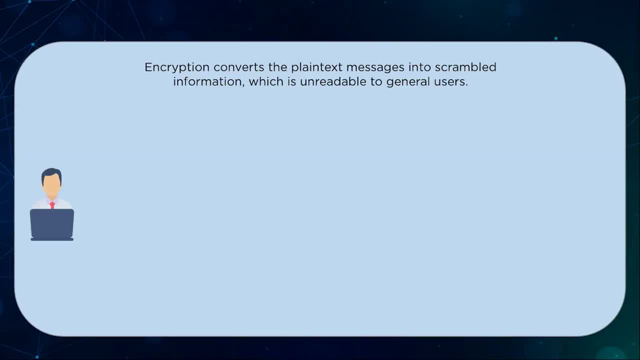 Encryption is the primary route for employing cryptography by adding certain algorithms to jumble up the data. Decryption is the process of reversing the work done by encrypting information to make it readable again. Both of these methods form the basis of cryptography. Any data pre-encryption is called plaintext or cleartext To encrypt the message we use. certain algorithms that allow us to decrypt the message. These methods are called plaintext or cleartext. To encrypt the message, we use certain algorithms that allow us to decrypt the message. These methods are called plaintext or cleartext To encrypt the message we use. 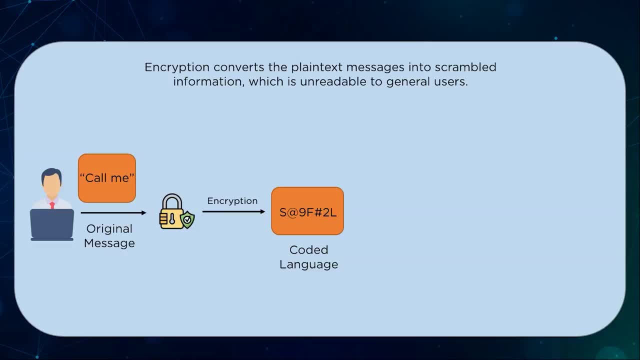 certain algorithms that allow us to decrypt the message. These algorithms provide an iterative response and are not necessarily a tactic, but they serve a single purpose of scrambling the data to make them unreadable without the necessary tools. They are a set of detailed steps to be carried out one after the other so that the data becomes scrambled. 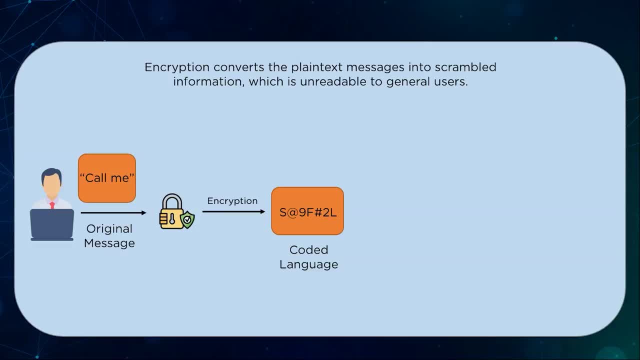 We take the plaintext, pass it through the algorithm and get the encrypted data. It is a coded language, which is also known as ciphertext, and this is the message that is transferred between both parties. The key being used to scramble the data is known as. 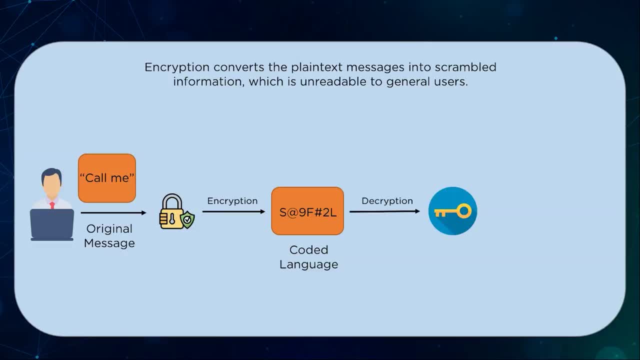 an encryption key. These steps and the encryption key are then made known to the receiver, who can use them to decrypt the ciphertext back to the original message. Unless any third party manages to find out the algorithm and the key used, they cannot decrypt the message. 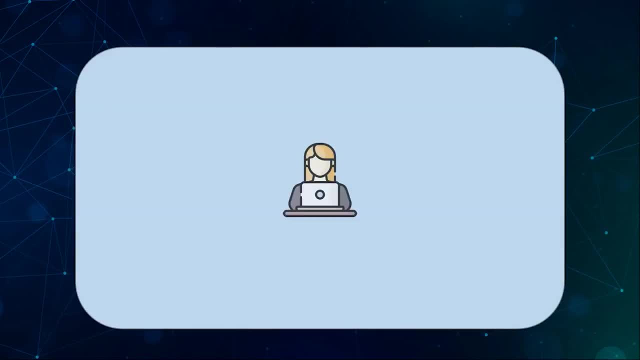 To put it as an example, let's consider Mary here. She wants to send the message call me today in an encrypted format, So this message becomes a plain text or clear text. We pass this string through an encryption algorithm that employs an encryption key to. 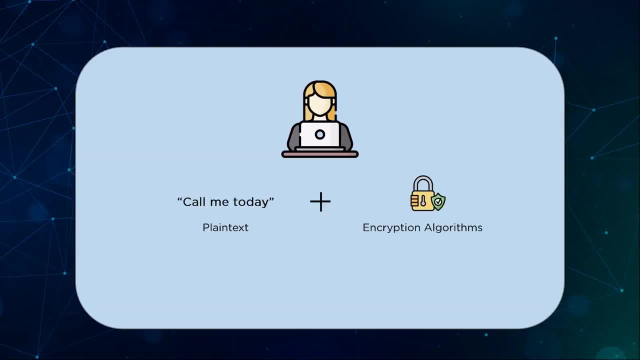 strangle the message. It makes it completely unrecognizable when compared to its original meaning. This is the ciphertext. The entire premise of encryption is to make this ciphertext as random and difficult to reverse engineer as possible. This ciphertext is then sent to Joe, who is the intended receiver for the message. 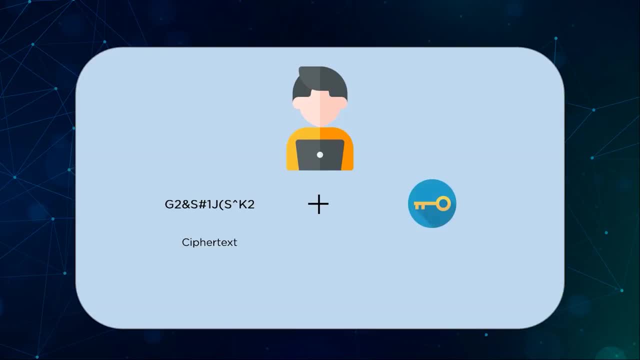 The ciphertext needs to be decrypted now using a decryption key. This decryption key is used to decrypt the message. This decryption key is the same as encryption key in some cases, while in other scenarios the keys are drastically different. Once the key is passed through the ciphertext, we can get the original message Mary intended. 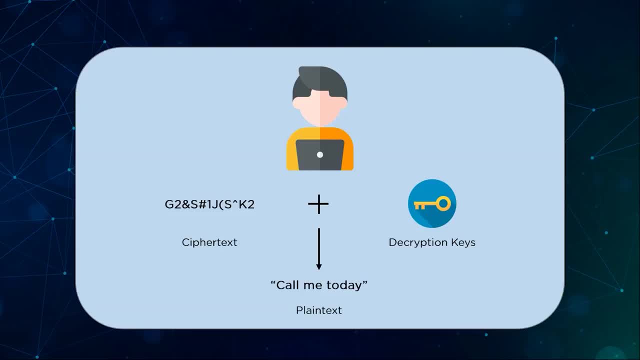 to send, which is the string: call me today. At no point in time did we lose any messages in transit, which satisfies the need for encryption and cryptography in general. Regarding the keys, we have two variants of key pair systems, one being the symmetric. 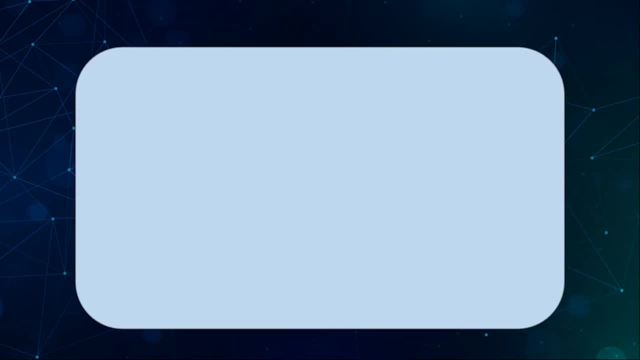 encryption and the other asymmetric encryption. In the former's case, a single key is used for both the encryption and decryption of data. It is comparatively less secure than asymmetric encryption, but it is much faster, which is a compromise that has to be embraced to deliver data as fast as possible without leaving the 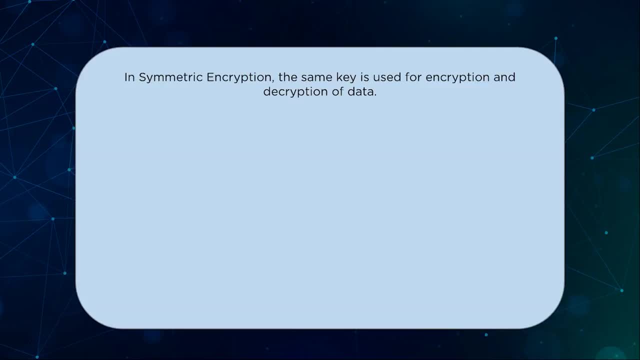 information completely vulnerable. This type of encryption is used when data rests on servers and identifies personnel for payment applications and services. We take up plaintext. We encrypt it first at the sender's site before transmitting it to the receiver. The receiver must have this key before he or she receives the ciphertext. so the original. 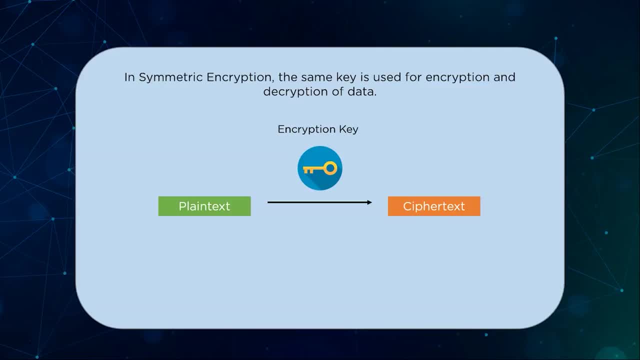 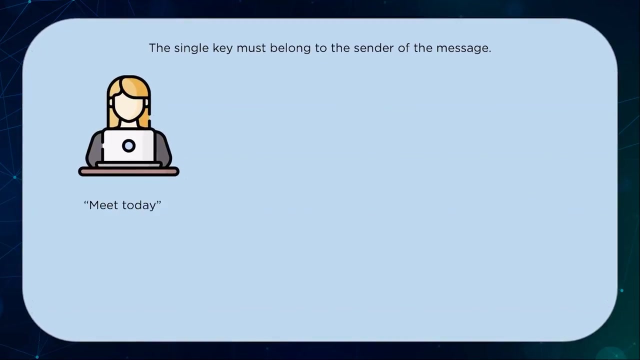 message can be recovered using this key. Another crucial aspect of this message is that the key must belong to the receiver at all times. If Mary wants to send a message to Joe with the message meaning meet today, the encryption key must be sent from her site first. 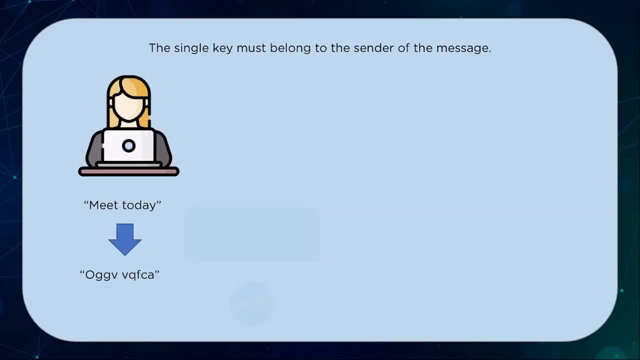 If Mary wants to send a message to Joe with the message meaning meet today, the encryption key must be sent from her site first. Once the message is encrypted using Mary's key, the ciphertext is then sent to Joe, who uses the same key employed to encrypt the message to decrypt the original ciphertext. 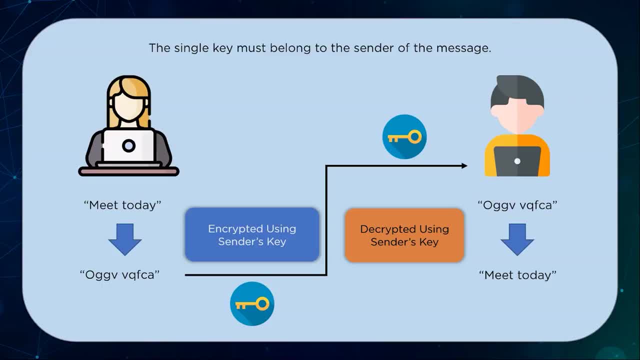 The potential drawback with symmetric encryption is that both the sender and receiver need to have the same key and it should be kept secret at all times. Caesar, Cipher and Rigmar Machine are both symmetric encryption examples. Cipher and Rigmar Machine are both symmetric encryption examples. 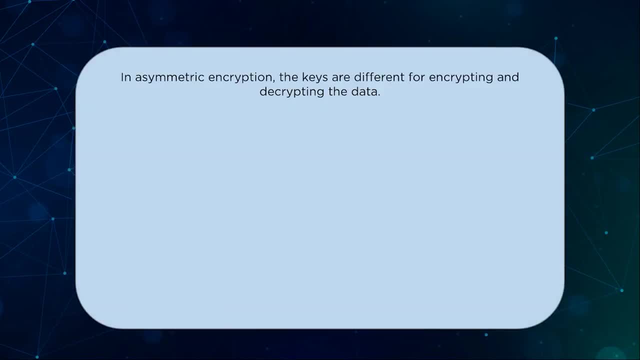 Cipher and Rigmar Machine are both symmetric encryption examples. Asymmetric encryption, on the other hand, has a double whammy at its disposal. There are two different keys at play here, a private key and a public key. A public key is used to encrypt the data pre-transit, and the private key is used to decrypt the. 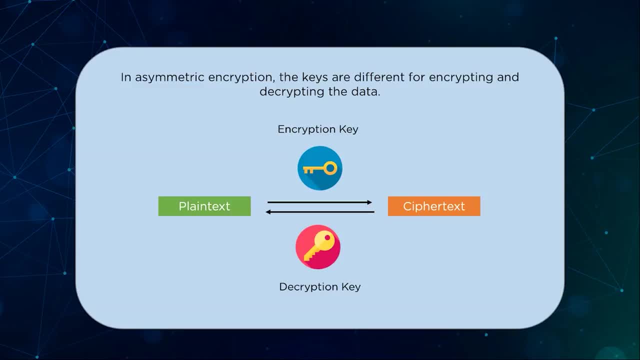 data post-transit. The ciphertext must be generated with one key and decrypted with another. ciphertext must be generated with one key and decrypted with another. Unlike its counterpart, both the keys in asymmetric encryption must belong to the receiver of the ciphertext. ciphertext must be generated with one key and decrypted with another. 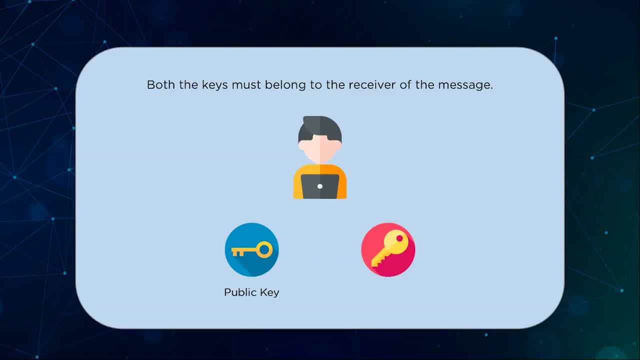 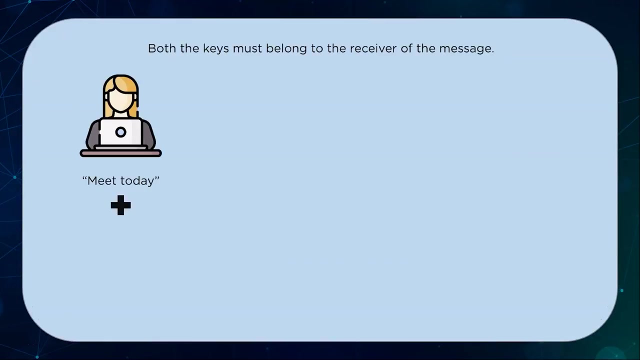 of the message. The public key used for encryption and the private key used for decryption must both belong to Joe, as in our example. To highlight the difference in execution for the same problem, let's say Mary wants to send the same meet me message to Joe. To encrypt the original plaintext she will need to use Joe's. 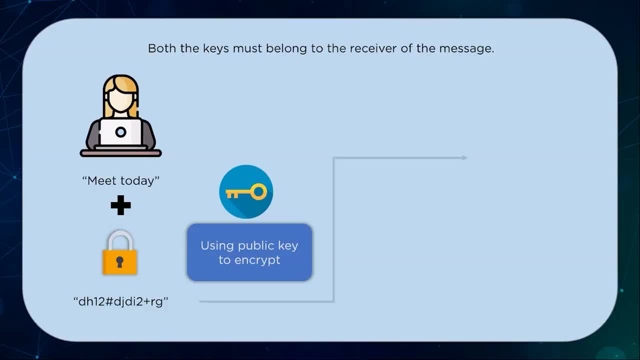 public key. Once the key is applied, the ciphertext is then sent over to Joe, who can use his own private key to decrypt the message so that he can receive the original message that Mary wants to send. This way, nobody can intercept the message in between transmission and there is no need for any secure key. 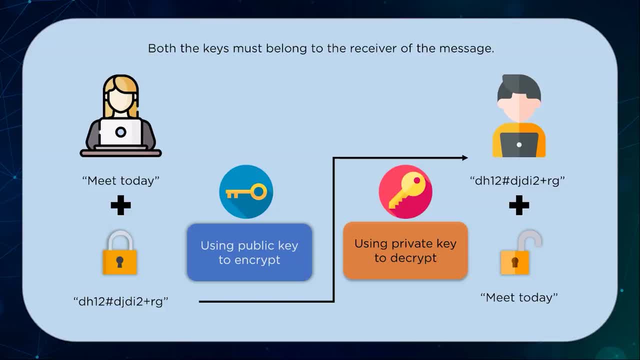 exchange. for this to work, since the encryption is done with the public key, Both the keys are necessary to read the full message. We may have understand now the necessity of encryption, but where do we use it in practice? Probably the most ingenious implementation of encryption is to use the private key to decrypt the. 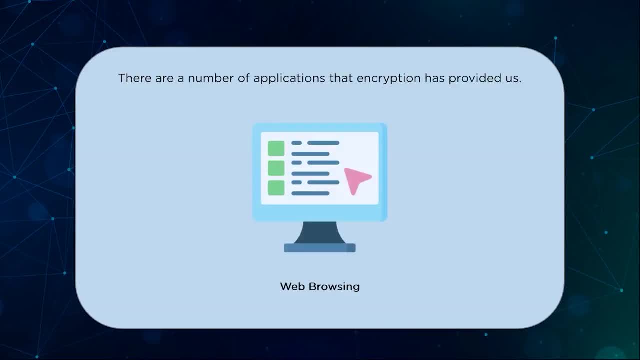 message. The secret to encryption is in our web browsing sessions. We can use symmetric and asymmetric encryption combined to monitor SSL or TLS encrypted browsing sessions to make sure nobody can steal our personal information. It plays a significant role in verifying website server authenticity and exchanging the 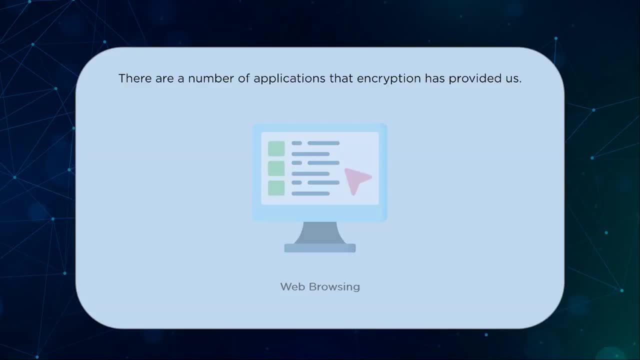 necessary encryption keys required. Apart from this, all the chat messaging applications we use nowadays, from Facebook to WhatsApp, employ encryption at some the architecture. This is a very controversial segment when it comes to IT data protection, since private messages hold critical information and have been proven to be instrumental in scamming. 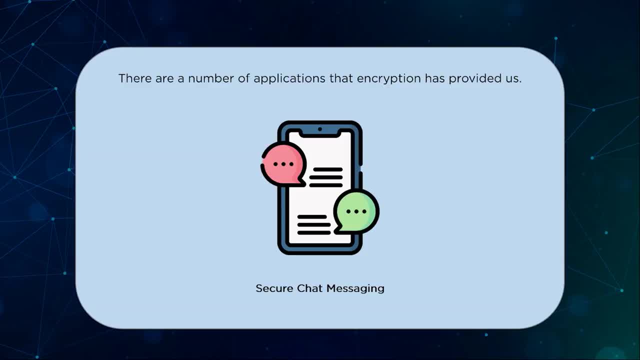 people out of their finances. A good encryption algorithm with solid key structure goes a long way in ensuring a safe and secure platform. Before the advent of chat applications, though, emails were all the hype, That doesn't mean they were left out in the security department either. 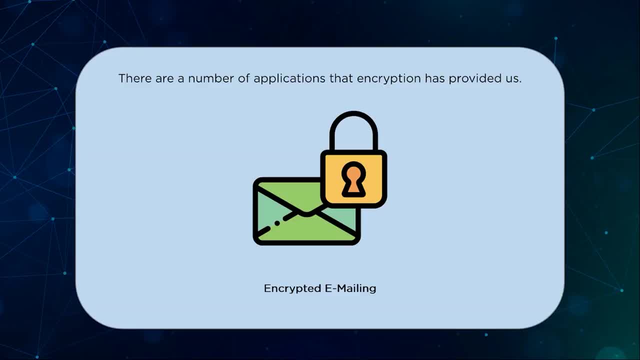 All email transfers are encrypted using algorithms that only the mail handlers, like Gmail, Yahoo and Hotmail, can decrypt. This allows a seamless experience for professionals and general public alike, who need to conduct most of their business via emails. Online banking applications also form a very important part of our convenience today, Starting from wallet apps like Paytm and Skrill. 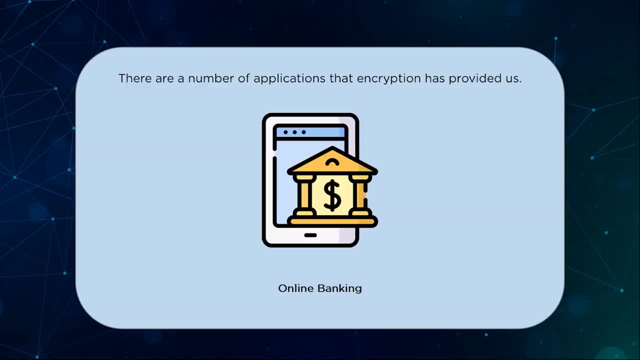 to specific net banking applications. encryption finds use. in encrypting online banking applications, We use our account details and transactions to prevent prying eyes from snooping on our data- A crucial part of any country's economy. banking application security needs to be audited on a 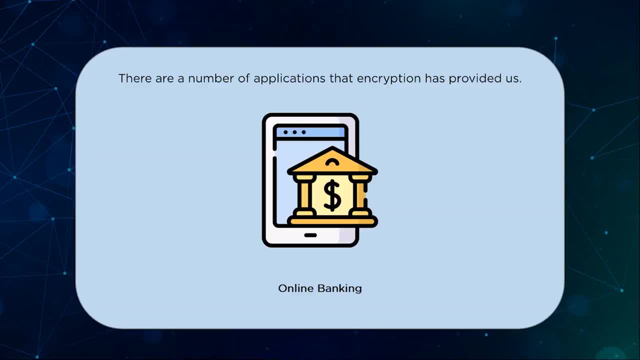 regular basis so that they can stay updated with the latest security patches and threats. Let's take a look at how our data is protected while browsing the internet thanks to cryptography. Here we have a web-based tool that will help us understand the process of RSA encryption. 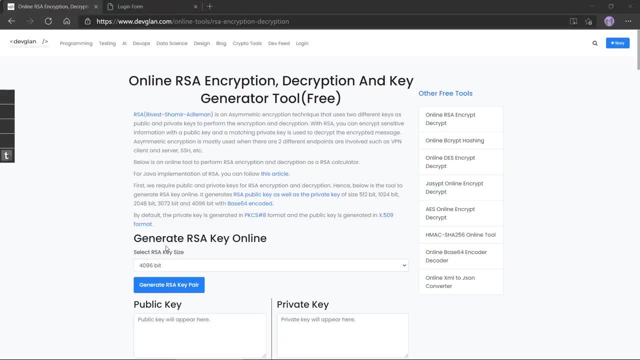 We see the entire workflow, from selecting the key size, which is the address of the number, and the time, which means the time for the message to be used, until the decryption of ciphertext in order to get the plain text back. As we already know, RSA encryption algorithm falls under the umbrella of asymmetric key cryptography. 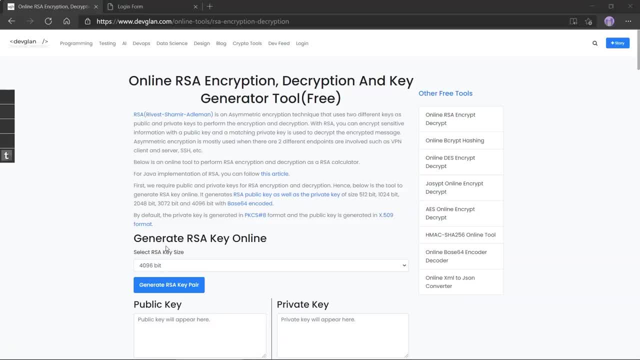 That basically implies that we have 2 keys at play here, a public key and a private key. Typically, the public key is used by the sender to encrypt the message and the private key is used by the receiver to decrypt the message. There are some occasions when this allocation is reversed, and we will have a look at that later. The second key is the SMS key, which is the sender key. This is the key that sends the message, and the receiver key is the decrypter key. There are few occasions when this allocation is reversed and we will have a look at that later. 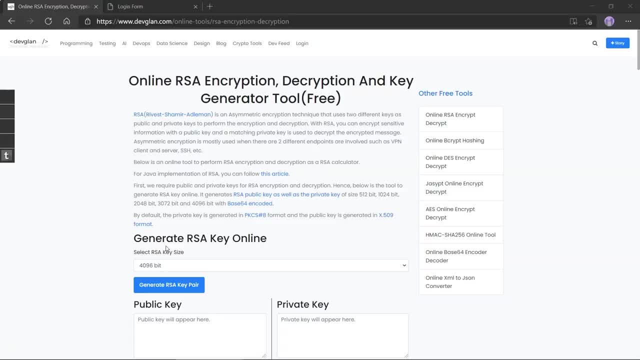 at them as well. In RSA we have the choice of key size. We can select any key from a 512 bit to 1024 bit, all the way up to a 4096 bit key. The longer the key length, the more complex the. 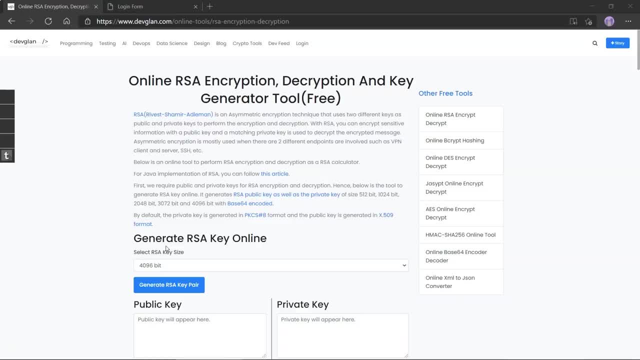 encryption process becomes, and thereby strengthening the ciphertext, Although with added security, more complex functions take longer to perform the same operations on similar size of data. We have to keep a balance between both speed and strength, because the strongest encryption algorithms are of no use if they cannot be practically deployed in systems around the world. 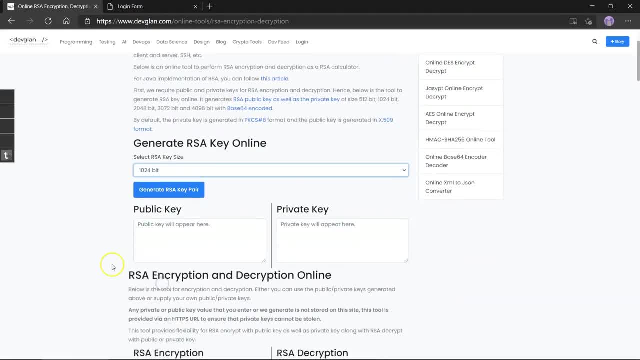 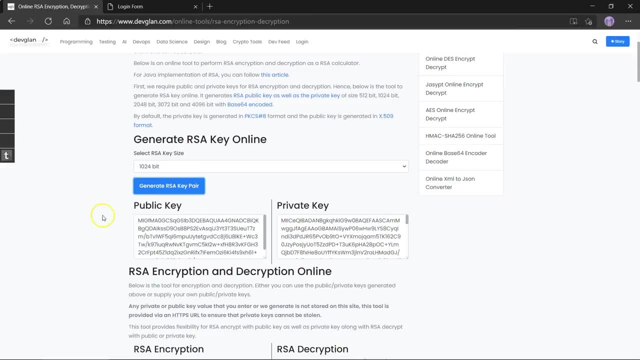 Let's take a 1024 bit key over here. Now we need to generate the keys. This generation is done by functions that operate on pass freezes. The tool we are using right now generates these pseudo random keys to be used in this explanation. Once we generate the keys, you can see the public key. 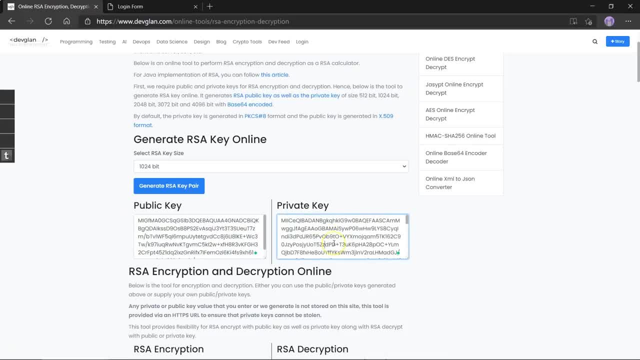 is rather smaller than the private key, Which is almost always the case. These two keys are mathematically linked with each other. They cannot be substituted with any other key and, in order to encrypt the original message or decrypt the ciphertext, this pair must be kept together. The public key is then sent to. 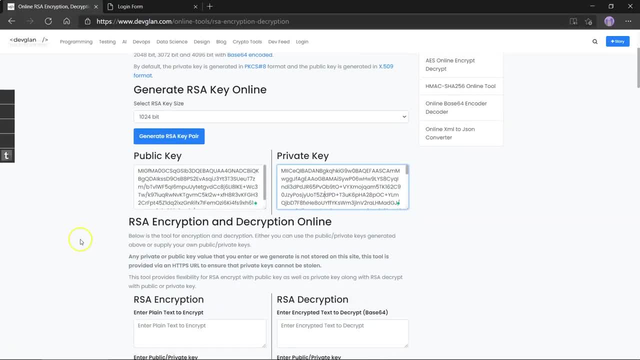 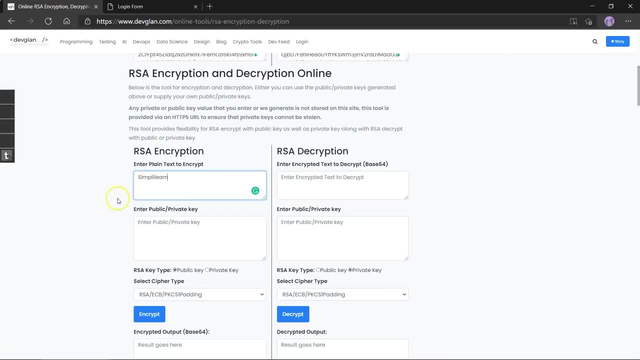 the sender and the receiver keeps the private key with himself. In this scenario, let's try and encrypt a word. simply learn. We have to select if the key being used for encryption is either private or public, since that affects the process of scrambling the information. 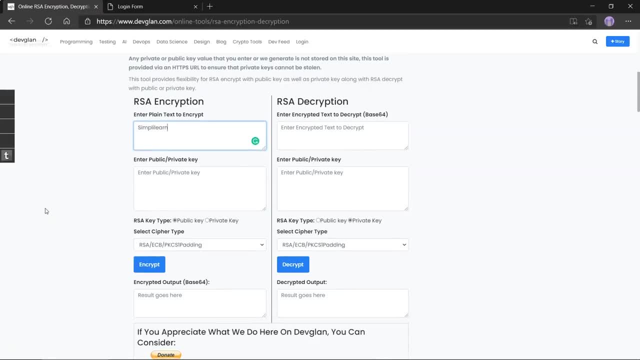 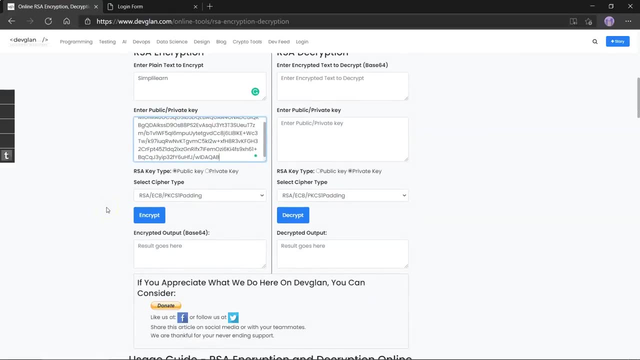 Since we are using the public key over here, let's select the same and copy it and paste over here. The cipher we are using right now is plain RSA. There are some modified ciphers, with their own pros and cons that can also be used. 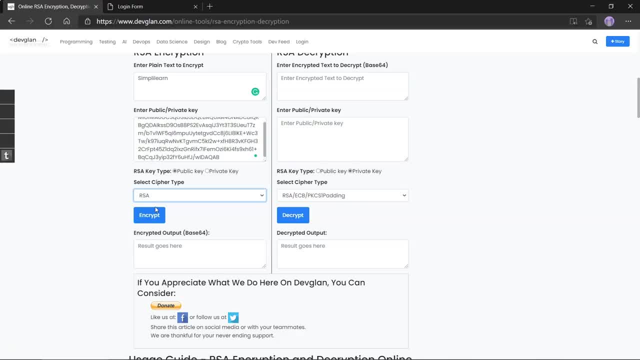 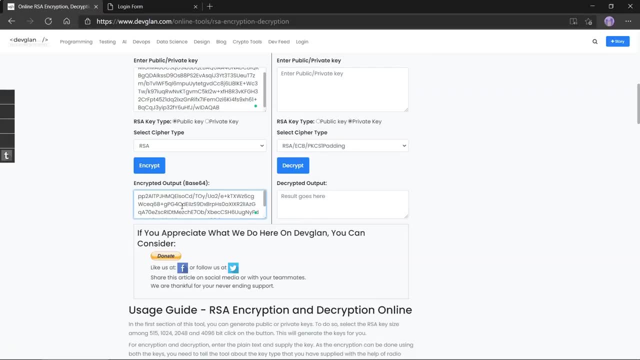 provided we use it on a regular basis and depending on the use case as well. Once we click on encrypt, we can see the ciphertext being generated. over here, The pseudorandom generating functions are created in such a way that a single character change in the plaintext will trigger a completely different ciphertext. This is a security feature to 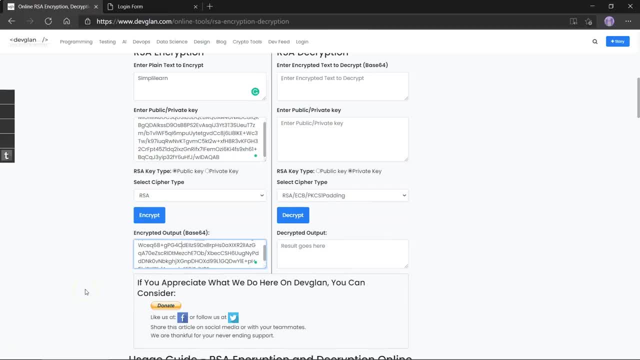 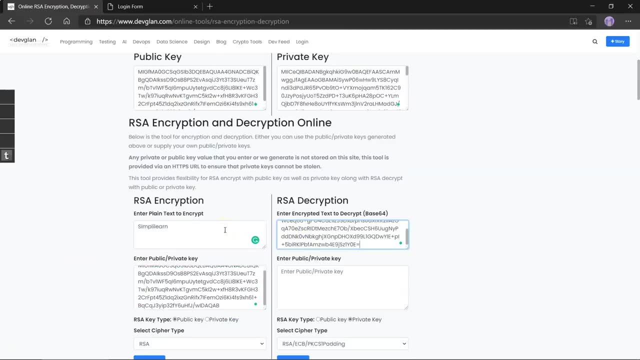 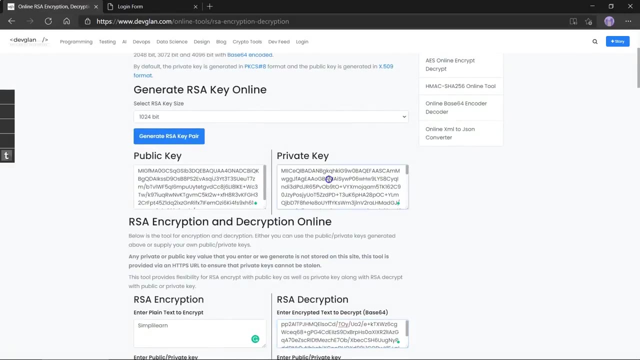 strengthen the process from brute force methods. Now that we are done with the encryption process, let's take a look at the decryption part. The receiver gets this ciphertext from the sender with no other key or supplement. He or she must inherently possess the private key generated from the same pair. 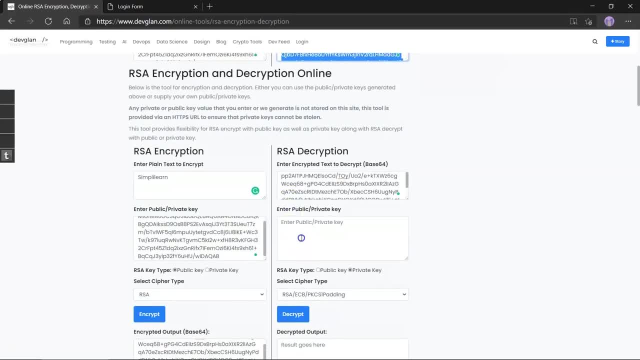 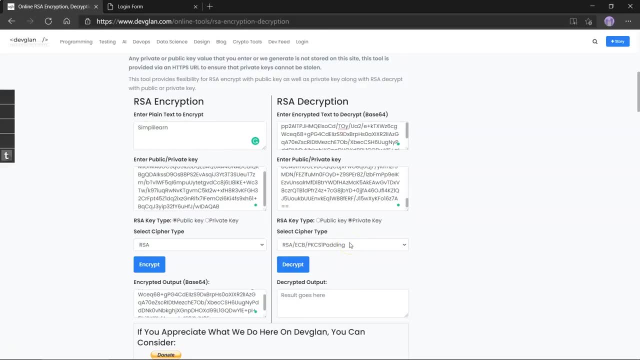 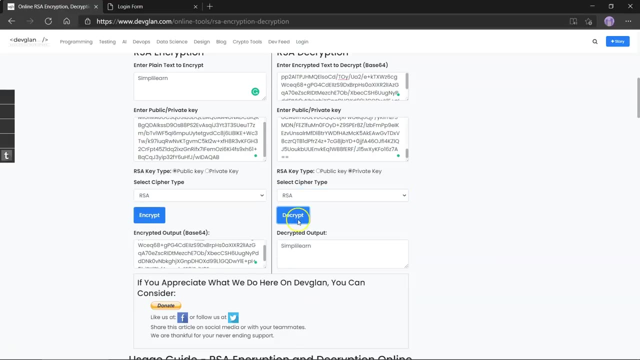 No other private key can be used to decrypt the message. since they are mathematically linked, We paste the private key here and select the same. The cipher must also always be the same used during the encryption process. Once we click decrypt, you can see the original plaintext we had decided to encrypt. 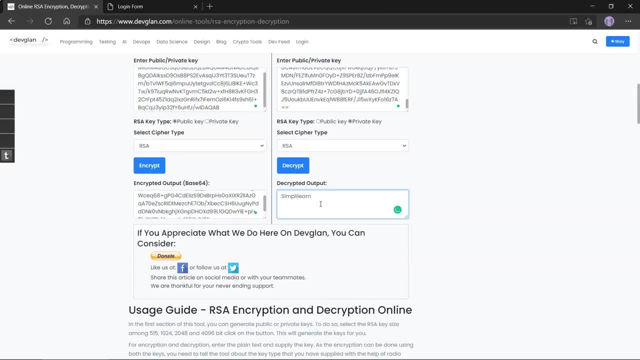 This sums up the entire process of RSA encryption and decryption. Now some people use it the other way around, also have the option of using the private key to encrypt information and the public key to decrypt it. This is done mostly to validate the origin of the message, Since 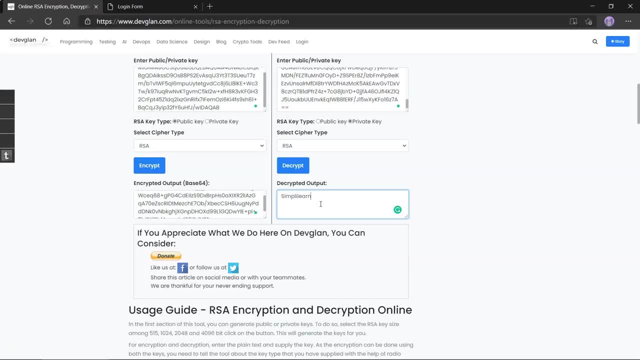 the keys only work in pairs. if a different private key is used to encrypt the message, the public key cannot decrypt it. Conversely, if the public key is able to decrypt the message, it must have been encrypted with the right private key and hence the rightful owner. 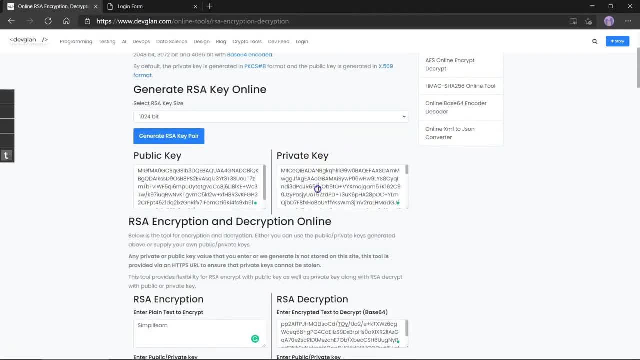 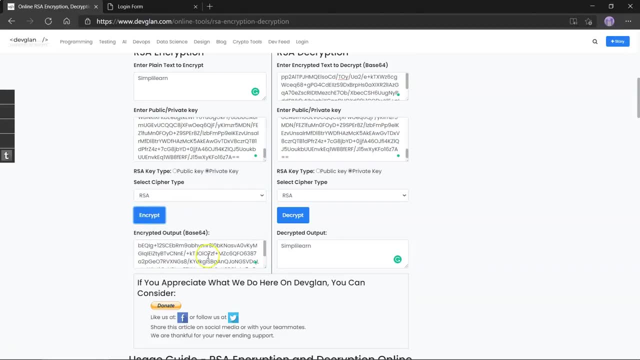 Here. we just have to take the private key and use that to encrypt the plaintext and select the same in this checkbox as well. You can see we have generated a completely new ciphertext. This ciphertext will be sent to the receiver, and this time we will use 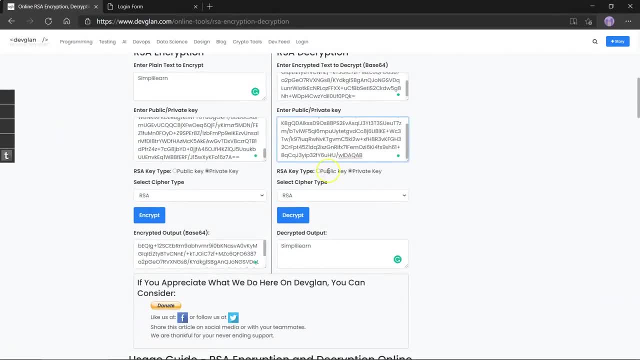 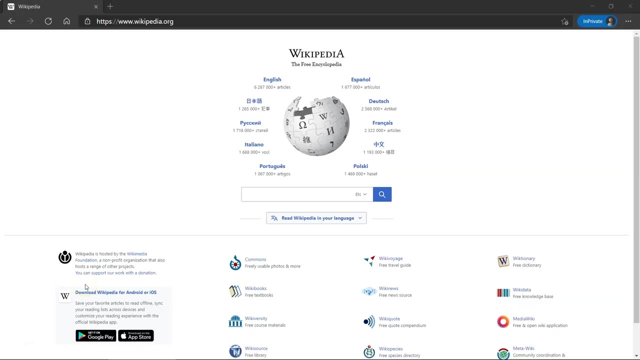 the public key for decryption. Let's select the correct checkbox and decrypt, and we still get the same output. Now let's take a look at practical example of encryption in the real world. We all use the internet on a daily basis and many are aware of the implications of using 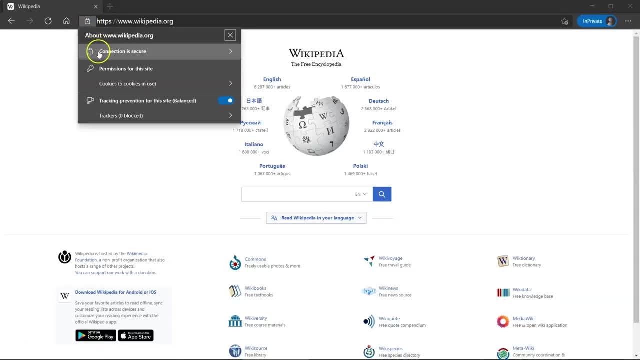 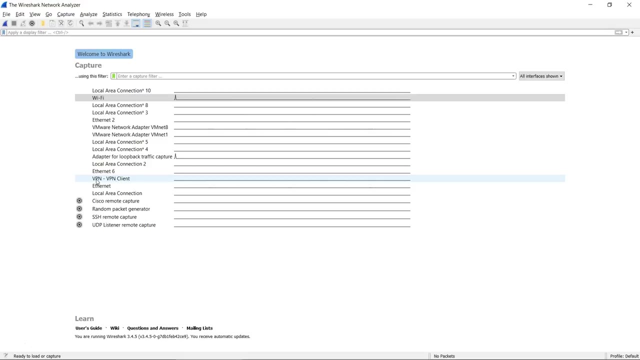 unsafe websites. Let's take a look at Wikipedia here. Pretty standard HTTPS website where the H stands for secured. Let's take a look at how it secures the data. Wireshark is the world's foremost and most widely used network protocol analyzer. It. 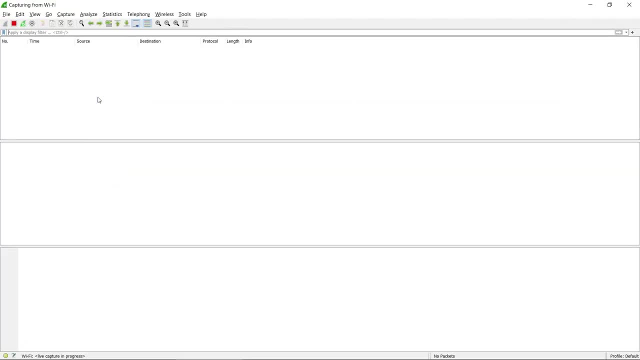 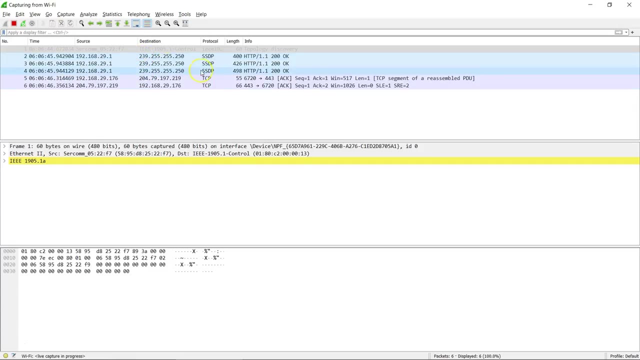 lets you see what's happening on your network at a microscopic level, and we are going to use this software to see the traffic that is leaving our machine and to understand how vulnerable it is. Since there are many applications running in this machine, let's apply a filter that. 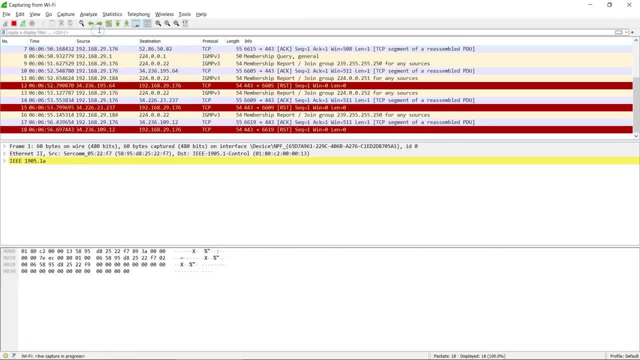 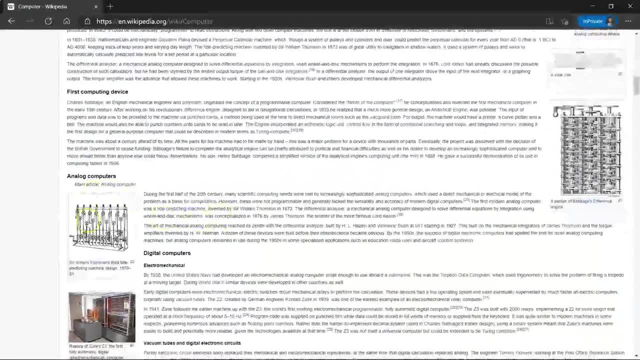 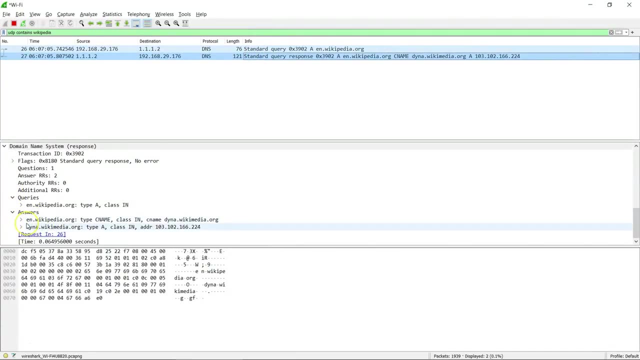 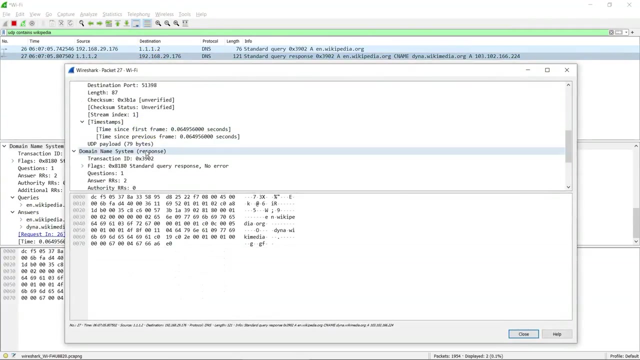 will only show us the results related to Wikipedia. Let's search for something that we can navigate the website with. Okay, Once we get into it, You can see some of the requests being populated over here. Let's take a look at the specific request. 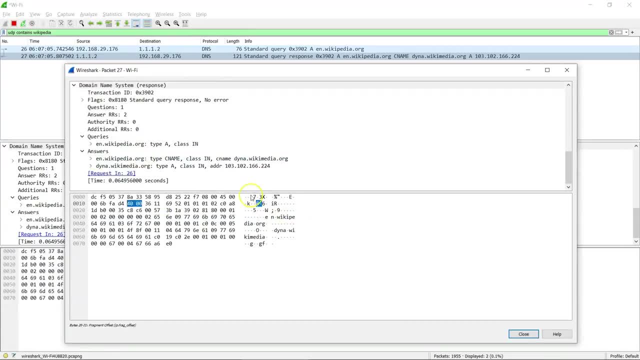 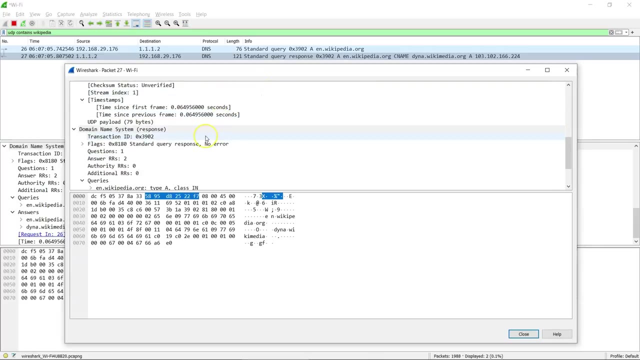 These are the data packets that basically transport the data from our machine to the internet and vice versa. As you can see, there's a bunch of gibberish data here that doesn't really reveal anything that we searched or watched. Similarly, other secured websites function the same way, and it is very difficult, if at 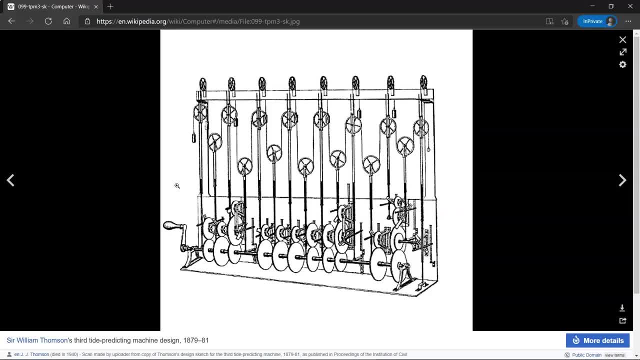 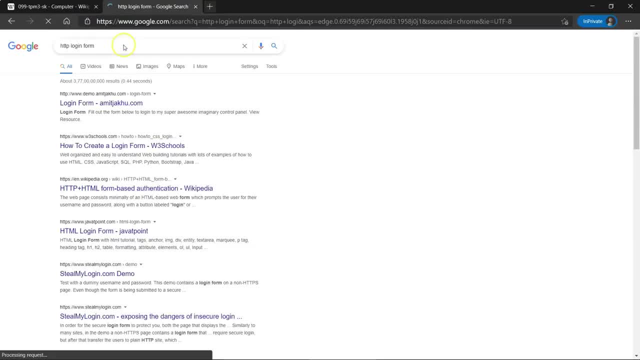 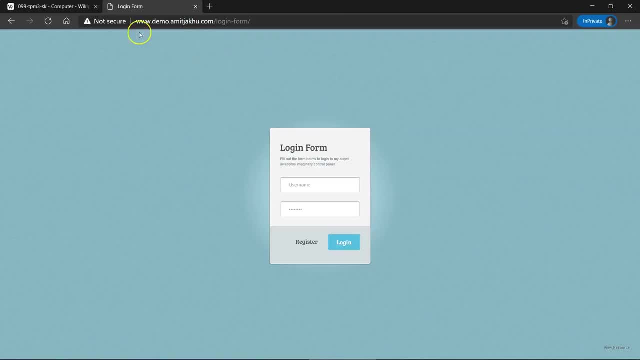 all possible to snoop on user data this way. To put this in perspective, let's take a look at another website, which is a HTTP webpage. This has no encryption enabled from the server end, which makes it vulnerable to attacks. There is a login form here which needs legitimate user credentials in order to grant access. 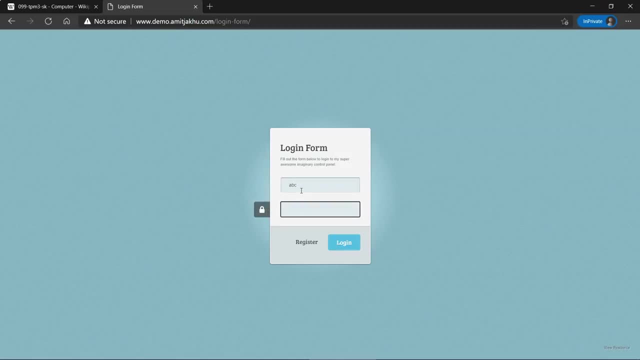 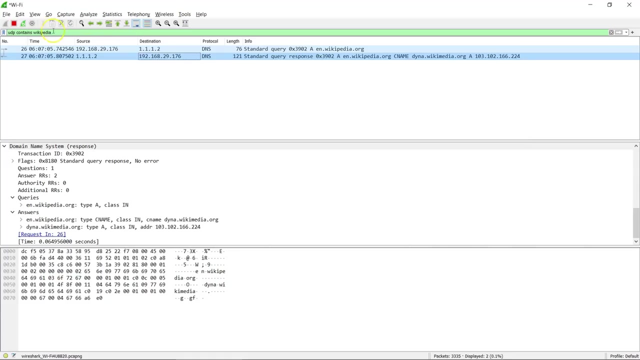 Let's enter a random pair of credentials. Okay, Let's enter a random pair of credentials. These obviously won't work, but we can see the manner of data transfer. Unsurprisingly, we weren't able to get into the platform. Instead, we can see the data packets. 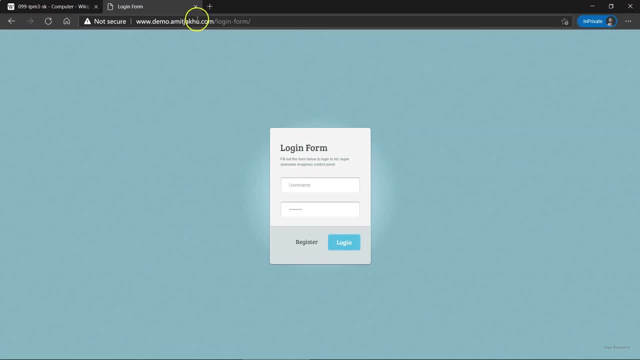 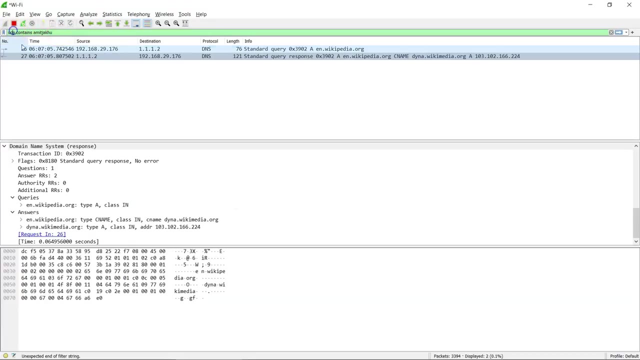 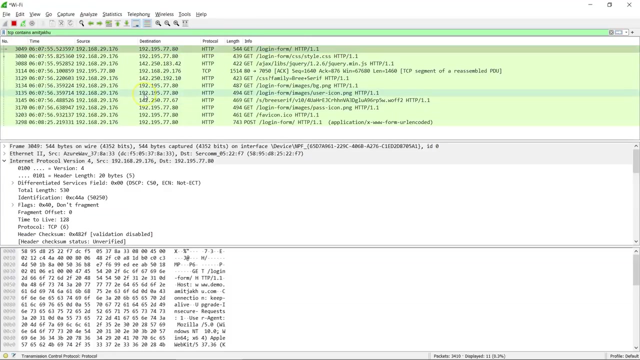 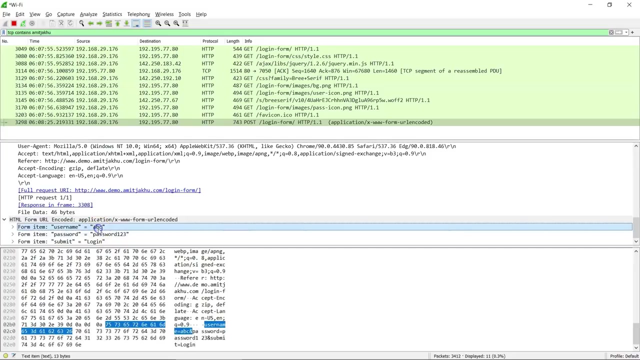 Let's apply a similar filter that will help us understand what request this website is sending. These are the requests being sent by the HTTP login form to the internet. If we check here, see whatever username and password that we are entering, we can easily 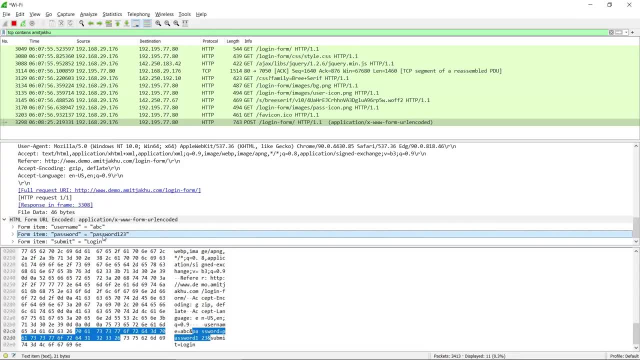 see it with the wireshark. Now, we used a dummy pair of credentials. Okay, If we select the right data packet, we can find our correct credentials. If any website had asked for our payment information or our legitimate credentials, it would have. 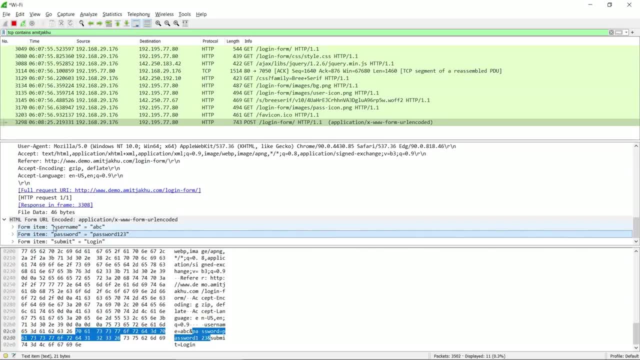 been really easy to get a hold of these. To reiterate what we have already learned, we must always avoid HTTP websites and just unknown or not trustworthy websites in general, because the problem we saw here is just the tip of the iceberg. Even though cryptography has managed to lessen the risk of cyber attacks, it is still prevalent. 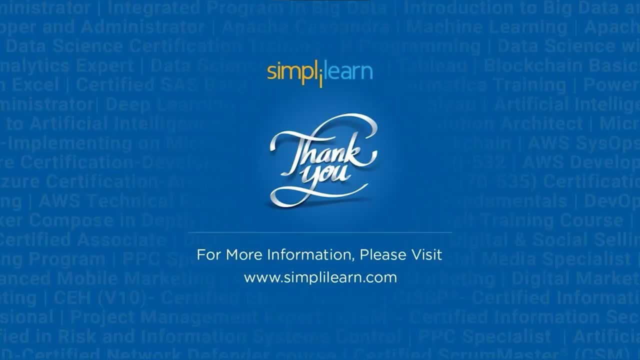 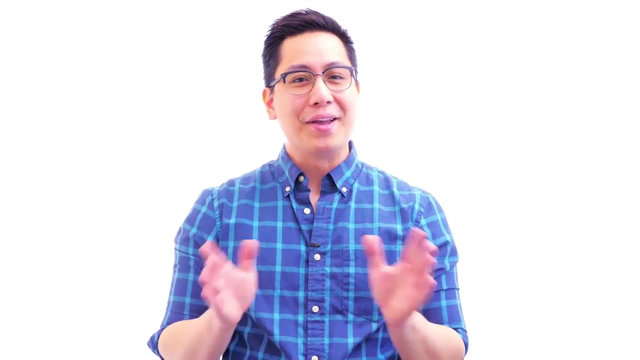 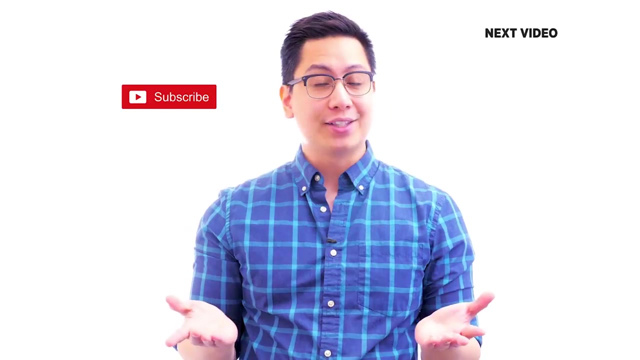 and we should always be alert to keep ourselves safe online. Hope you learned something interesting today. If you have any questions, please ask us in the comment section and subscribe to our channel for more videos like this. Thanks for watching.